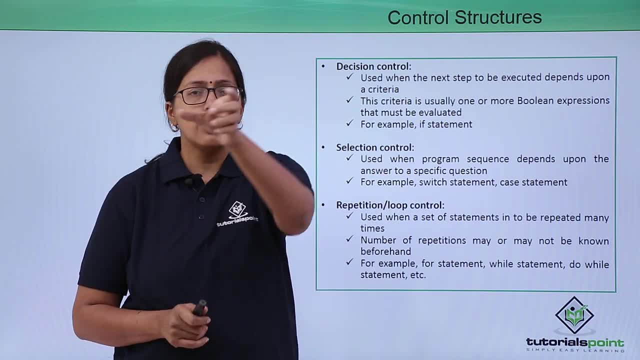 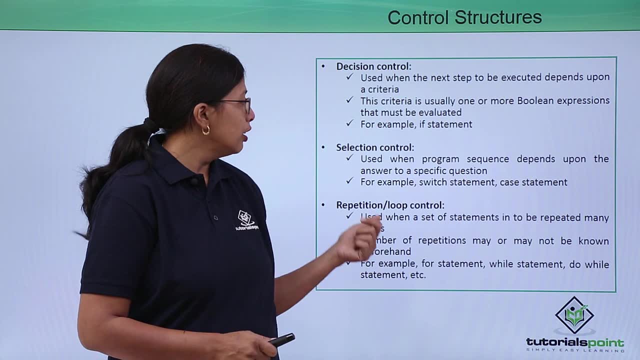 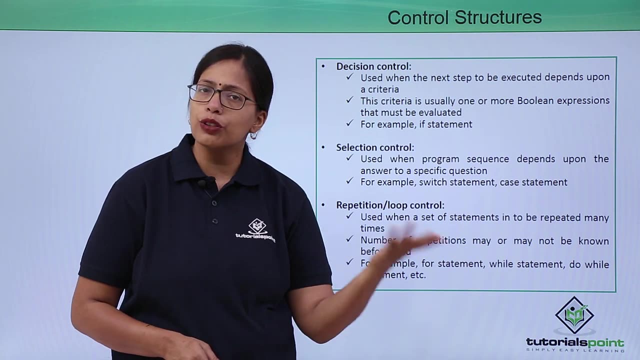 1, you have to follow these steps. If he selects 2, you have to follow these steps. If he selects 10, you have to follow these set of steps. So there the selection control structure is used. Example: switch statement. case statement. depending on the programming language you will. 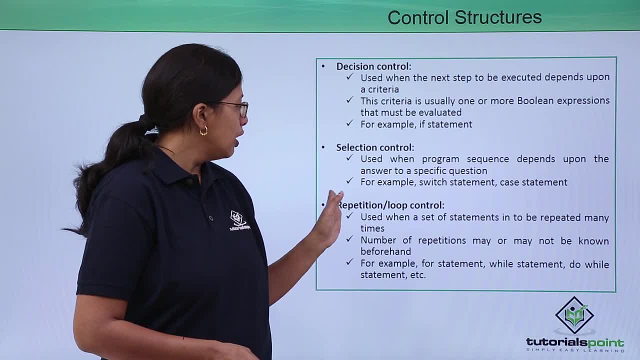 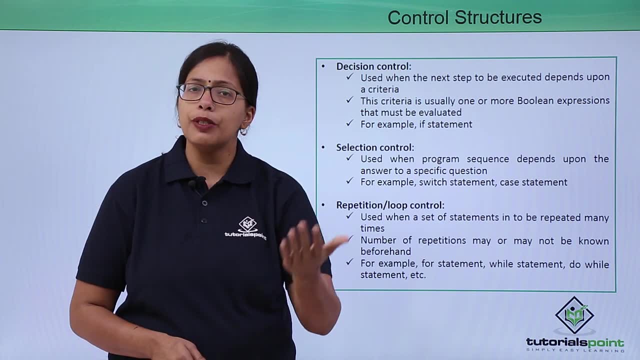 have different name for that control structure: Repetition or loop control. Always there will be some set of instructions that have to be repeated again and again. There the repetition control structure or the loop control structure is used because it is counterproductive. if you have to, 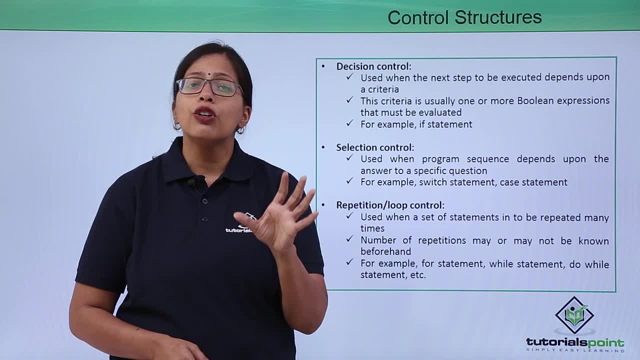 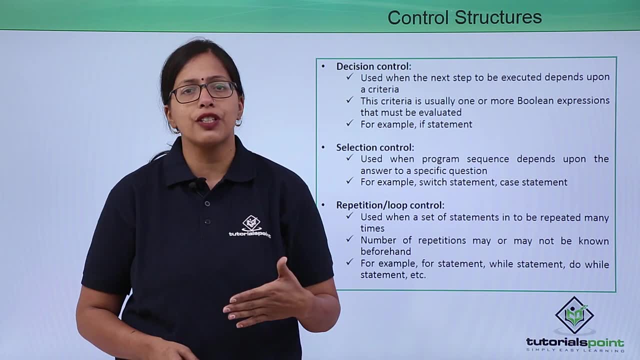 write it so many times. Also, you will have to know beforehand how many times the statements have to repeat it. This is not actually the case, So you have to know beforehand how many times the statements have to repeat it. scenario: In a real life situation, the user might tell you how many times it has to be. 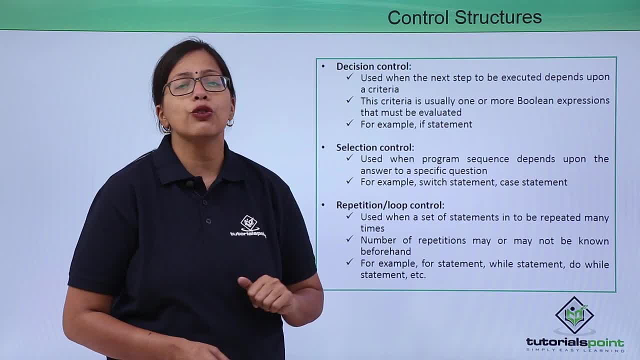 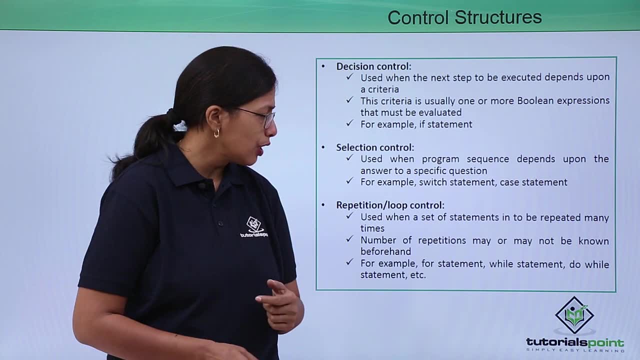 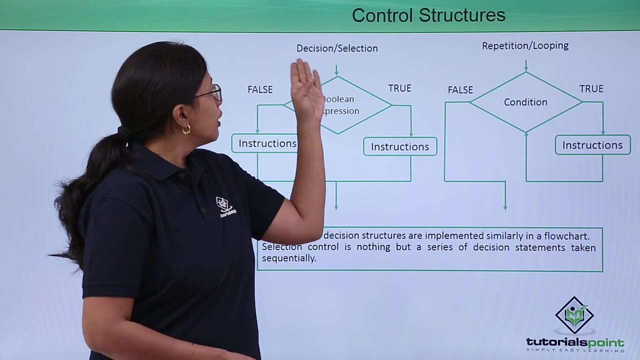 repeated. So in that case a loop control statement is used. Usually it is a for statement, but it will depend upon the programming language that you are using. Let me show the flow chart for the statements For decision or selection control. Boolean expression. If it is false. 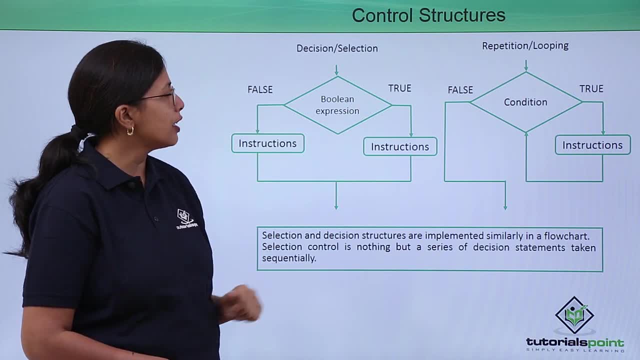 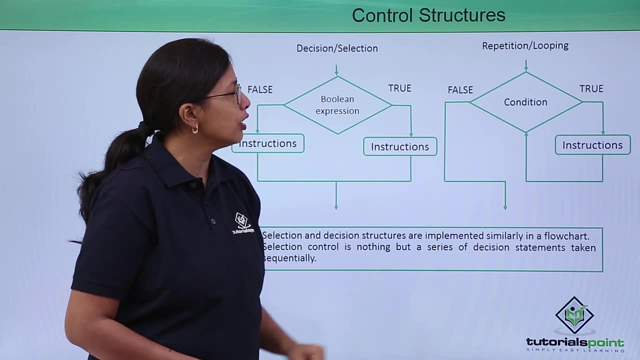 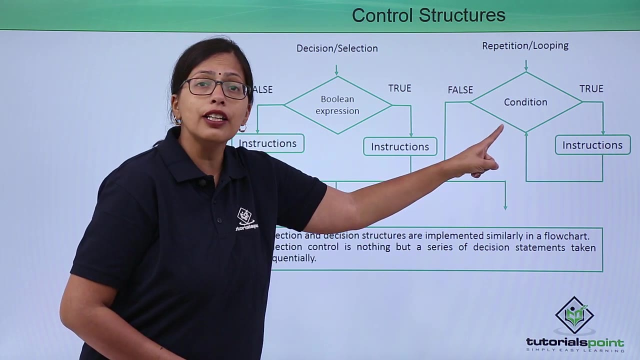 one set of instructions. If it is true under set of instructions. Now see the difference here In the repetition control structure. this is condition true. If it is true, these instructions will be repeated. You can see that it is going back to the condition. The condition is checked again. True: same set of instructions. 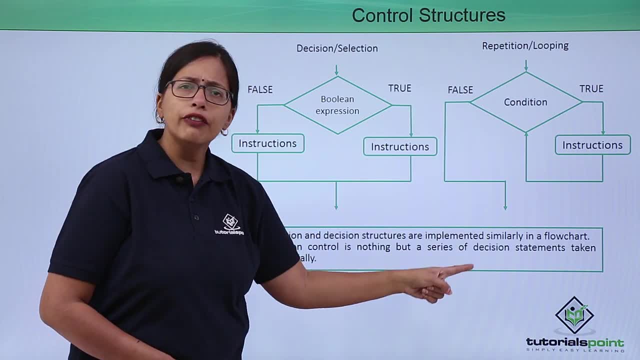 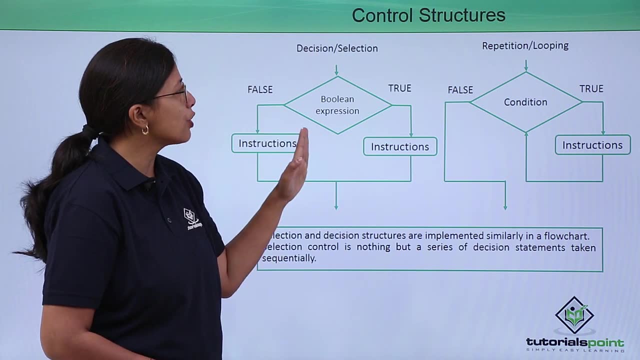 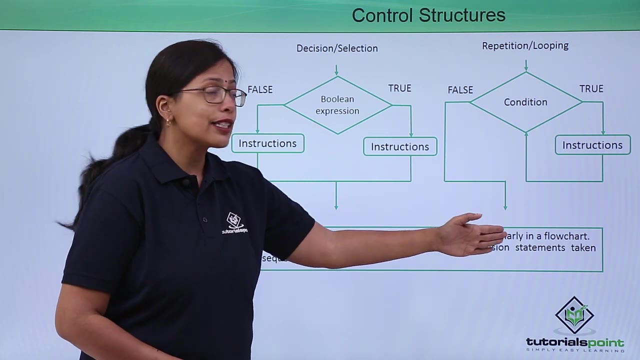 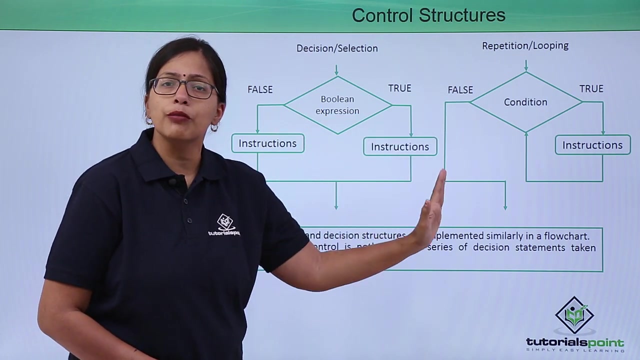 repeated. If it is false, then it will do some different set of instructions. So this is the control structure: Decision or selection and repetition. Selection and decision control structures are implemented similarly in a flow chart. This, this, this: You can see that we are using similar symbols. We will be discussing this.